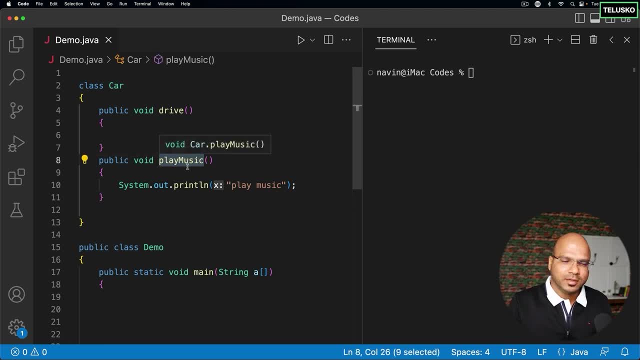 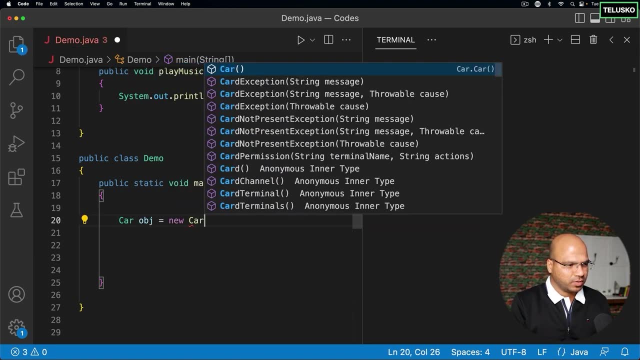 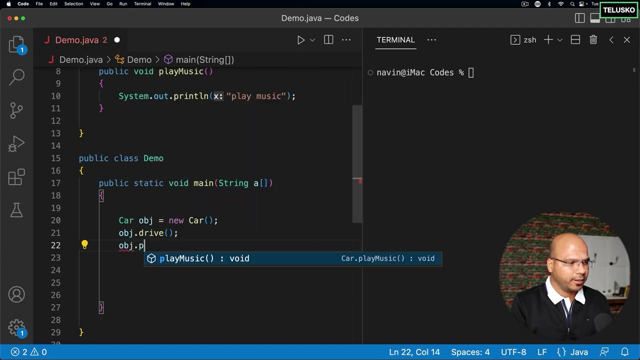 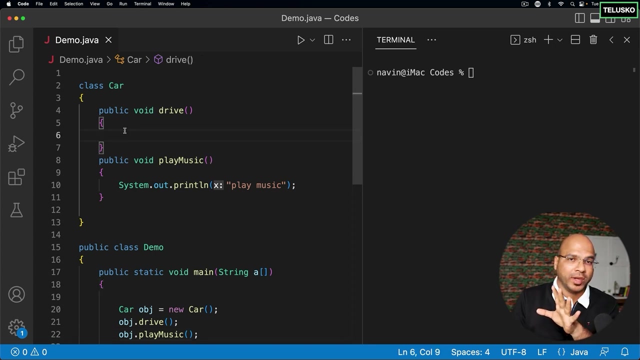 you will call it a car, you can state it's a home theater. Anyway, now if I want to use this car, I can simply create an object. I can say OBJ car, OBJ equal to new car, And then I can call the methods. I can call both the methods: OBJ dot drive and OBJ dot play music. Of course we have two methods, like I should be able to call them. Now, if you observe, in the drive we are not doing anything. why we're not doing anything? because I don't know how to implement drive, But I know how to implement play music, So I'm 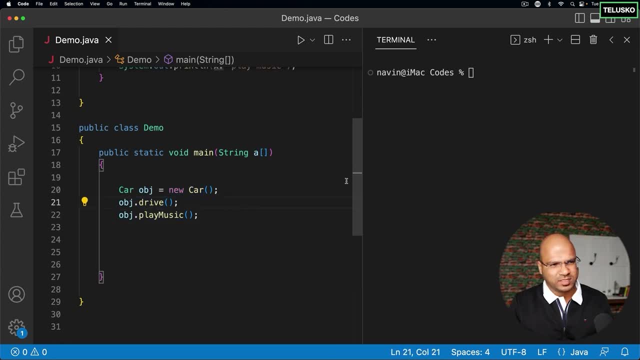 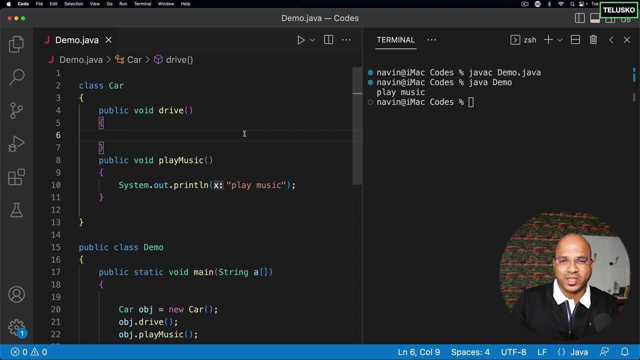 able to do that. I'm able to create this object and I'm able to call these two methods And I think it should work. And if I go back and run, it works. It's not like if you don't define something it will not work, it's working. The only thing is, when you're defining this method, you are actually not implementing anything here. you're not writing any statements, So it's valid in Java syntax term, But as a feature. I mean, just imagine you're buying a new phone and your phone says it can do this feature, this feature, feature one, feature two, feature three, but then none of the feature works, Of course. 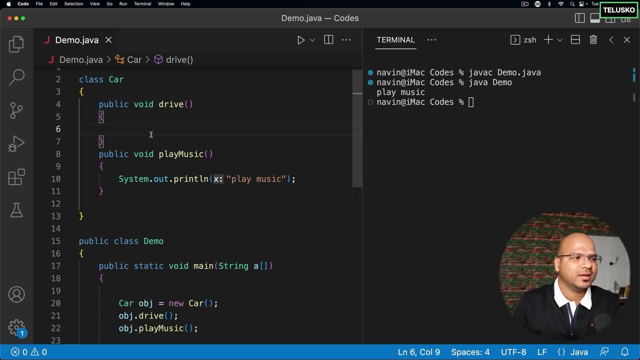 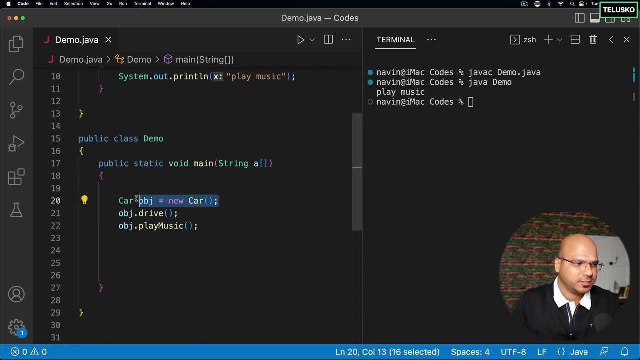 you will not buy any phone like that right. In the same way, if we talk about this car, you are writing a method over here which is drive, and you're not implementing it. Why someone should be able to create object of this? Why, in first place, someone should create a class itself? 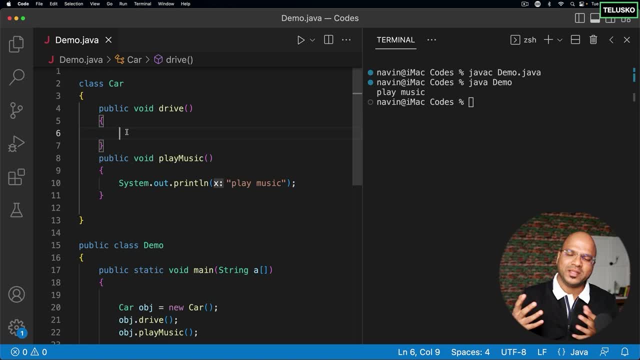 right when you don't know how to implement it. So the thing is, when you build an application, you have a structure which you follow. you design your application. not, I'm not talking about the thing you which you see on the screen. I'm talking about when you build an application. 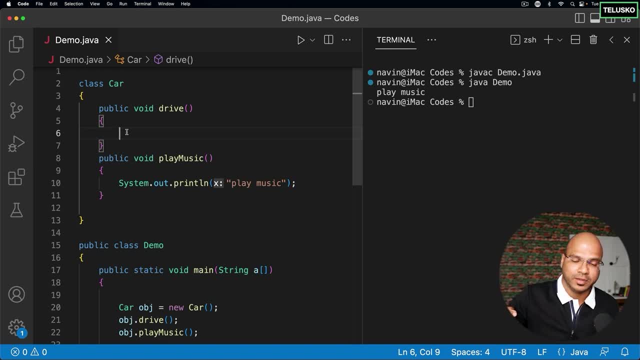 you design on paper. what are the classes you need, What are the methods you need? Now, at this point, you know how to play music, but you don't know how to drive. Now, in that case, should I remove this method completely? If I do that, then how will you call it as a car? 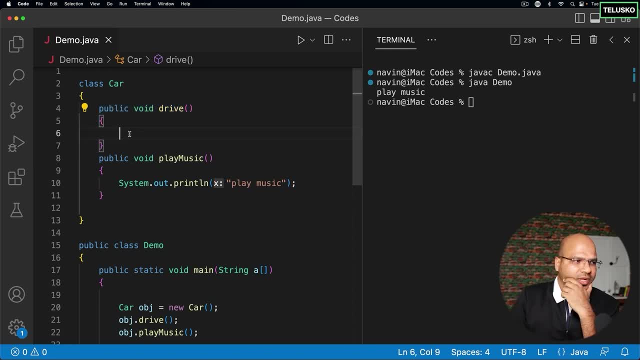 So what you can do is you can say: hey, you know I am creating this method drive, but I'm not sure what should I implement it here? So, instead of defining it here, so when you open the curly packets and close, you are basically defining a method. So, instead of defining a method, 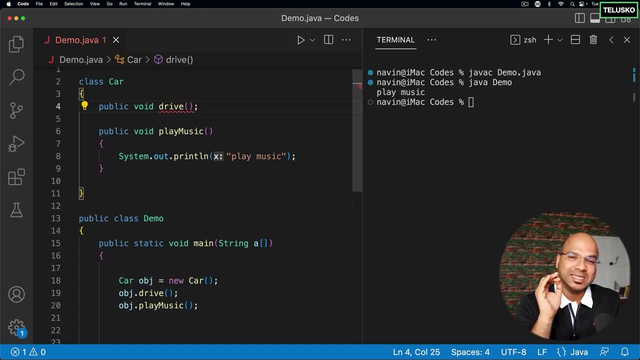 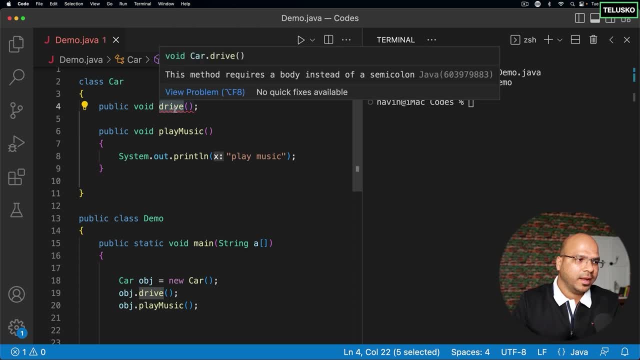 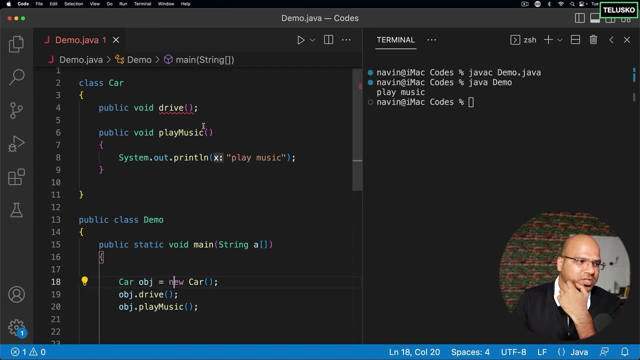 the drive feature you had declaring, but it is not working and no one should be able to create object of it. Okay, again, we'll see that in some time, But when I declare it it is giving you an error. Now, first of all, why you will declare when you are not defining anything. maybe I have 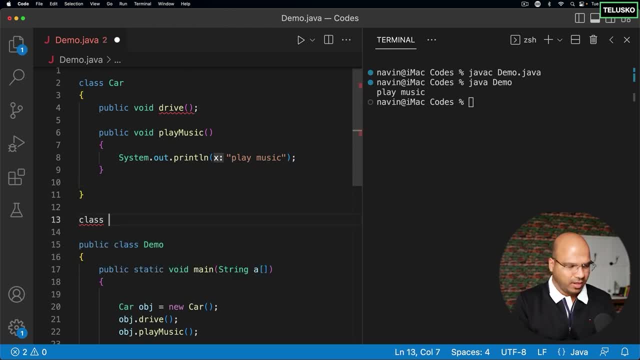 this mindset. someone else can just come back and they can say: they can implement a car, maybe they will build a wagon. let's say, and a wagon will extend my car and it is the wagon's responsibility. In fact, you know, instead of saying wagon. 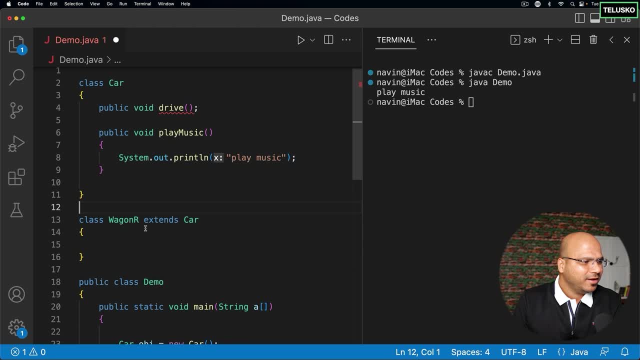 let's say WagonR. it's a very famous car if you search online. So we have this WagonR car, which some of them don't like, not a big fan of it, But okay. so let's say we have this car. 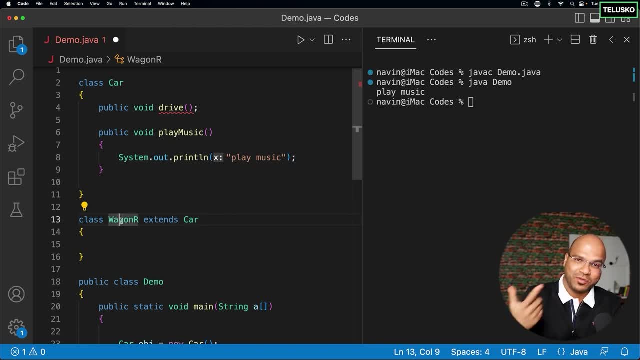 WagonR extends car. In fact, I have a car which is smaller than WagonR, which I love. So we have this class WagonR extends car here, And what I want here is: I want this WagonR to implement. 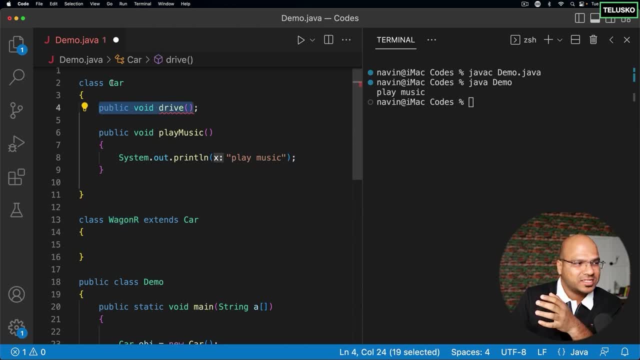 the drive feature. See, if you think car is just an abstract concept, right, No one actually buys a car. what you buy is a real car like WagonR or BMW GLS or Toyota Fortuner or Ford EcoSport- right, So you buy a real car. you don't buy a car, this is just a concept. So when I say: 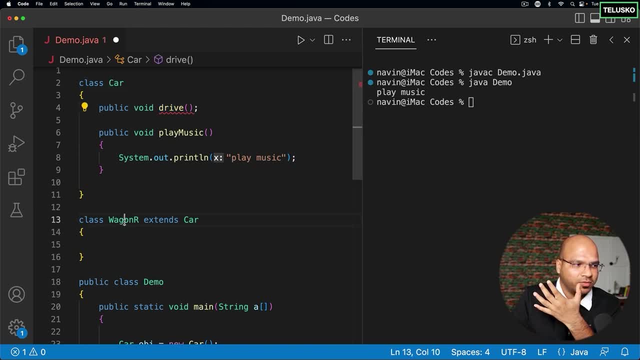 drive here a car don't know how to drive, But then when you, when you create a real car, that car will know how to drive. So I want this WagonR to be responsible to define this method, Because I can just copy this and paste it here And here instead of declaring it. I will define. 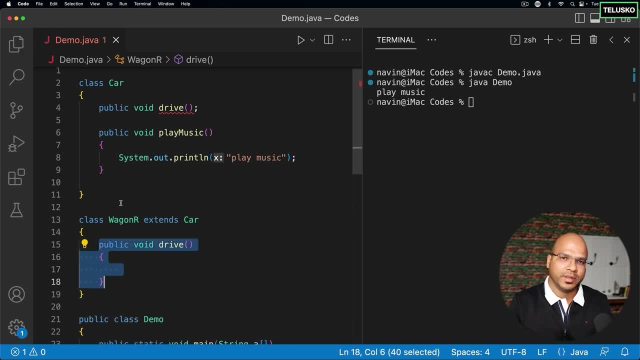 So what I want is: I want this WagonR to implement it. Of course, the other feature, like play music, can simply be extended, but not drive. Drive should be implemented here, And WagonR I mean the company who built WagonR cars. it's their responsibility to define the method here. I can. 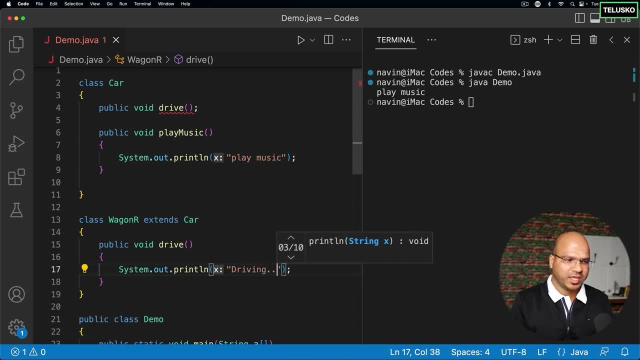 say, driving. of course, they will write a complex logic, But just to make it simple, I'm writing one particular thing that I want to implement in this particular case, which is I want to make it possible to define this method, and we're not doing it here Now. if you want to declare a, 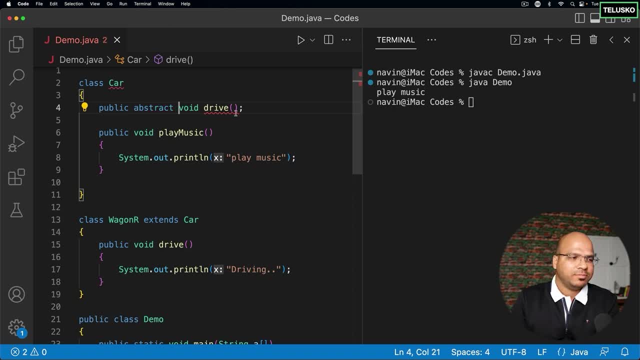 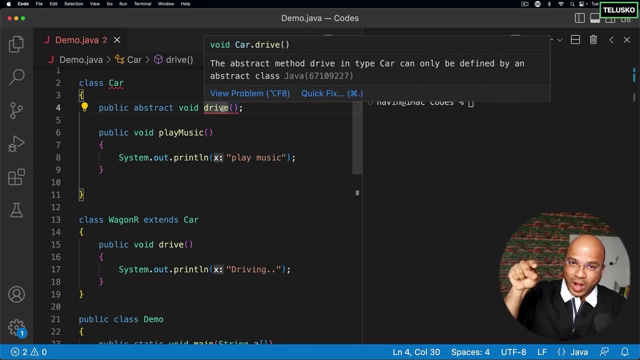 method. you can see we are getting an error here. you can use an abstract keyword, So when you say abstract, it means I'm just giving you the abstract idea of a car should have a drive feature, but I don't know how to implement it Now, when you are using my feature and when you call your vehicle, 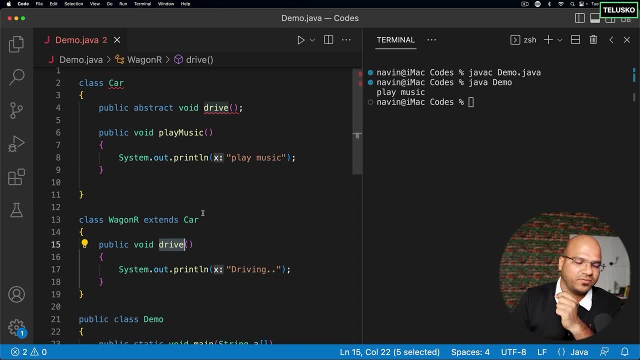 as a car, it should have a drive feature. Or whatever object you're creating is a car, you need to have a drive feature And that's how you make it possible to define the method. it, so you make a public abstract, void drive, so you have to use an abstract. 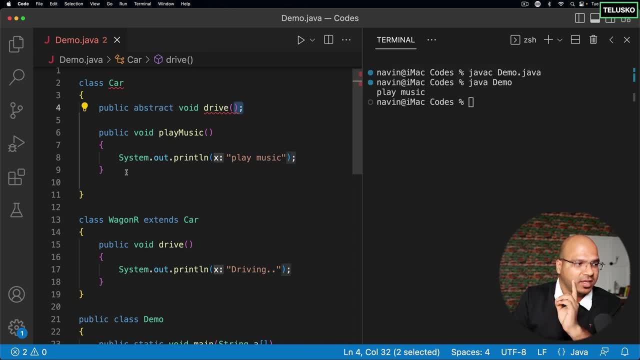 keyword. if you want to declare a method, okay, here we are defining it. but if you can see, even if I do abstract, it is giving you an error. it says the abstract method drive in type card can only be defined by an abstract class. okay, what it simply means is, if you have an abstract method, abstract method can. 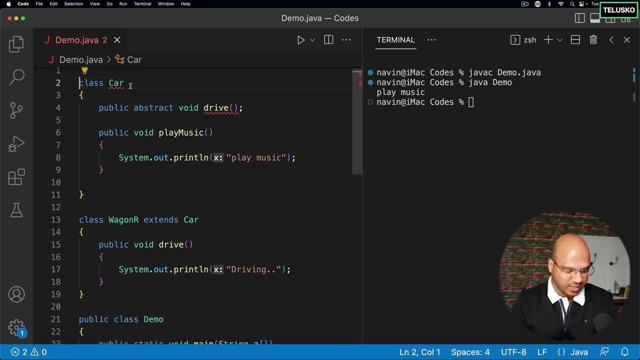 belong to only abstract class. so that means you have to make this class as abstract as well, so you can have abstract methods only in the abstract class. and whichever class is extending the abstract class will have this drive method. if we don't do that, it will give you an example if I change the method. 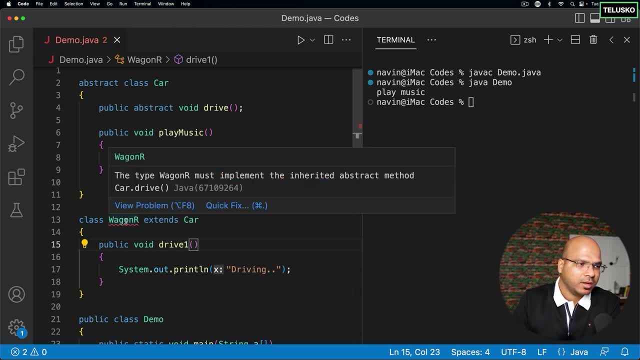 name you can see it will give you error. it says the type Wegener must implement the inherited abstract method car dot Drive. so if you are extending an abstract class you need to define it compulsory, otherwise it will not work. so you have to define, you have to basically overwrite the method. 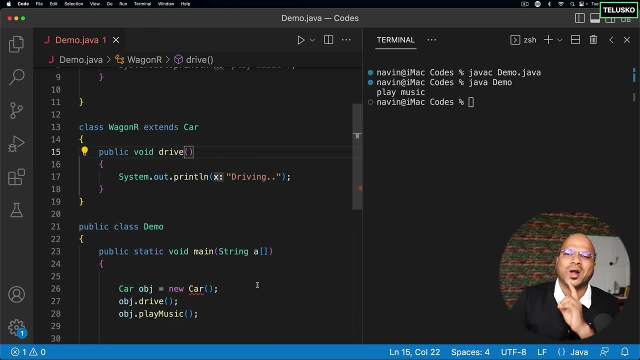 you have to define it compulsorily, otherwise it will not work. so you have to basically override the method. Now, when someone creates an object of a car, in fact, first of all you can't create object of abstract class Point, very important point. 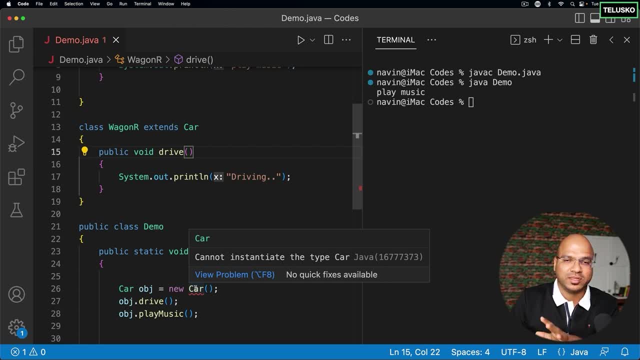 And that's why you can see we got an error here. It says: cannot instantiate the type car. It simply means you cannot create object of car. So the point remember: you cannot create object of an abstract class. Okay, but then can I create a reference of abstract class? 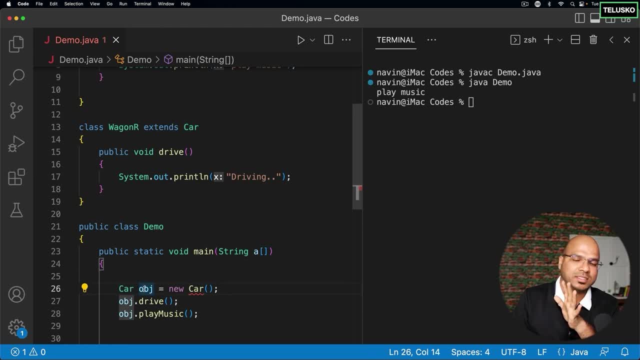 Yes, that is possible. You can say car obj, that is absolutely correct. But if you want to create an object you have to get object of not car but WagonR, okay, And then with this obj you can call drive. 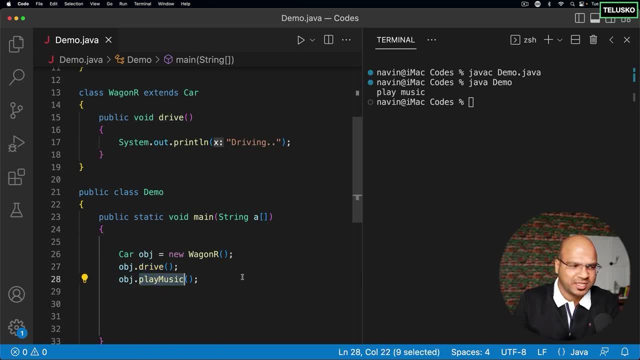 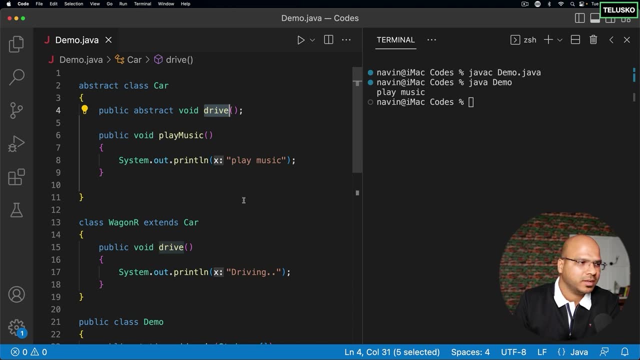 you can call play music, And we have talked about dynamic method dispatch And we know when you call drive, it will be calling drive of WagonR, not of car. Anyway, it is declared right. So basically, that's how you can create an abstract class. 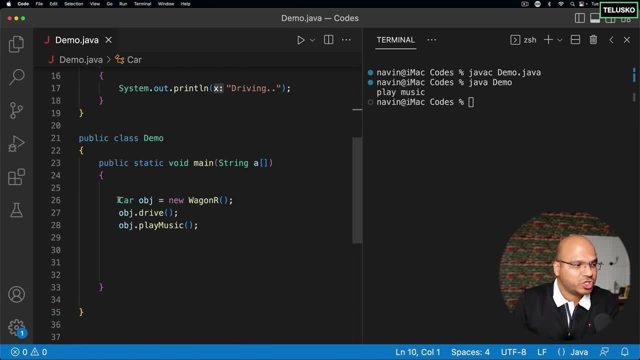 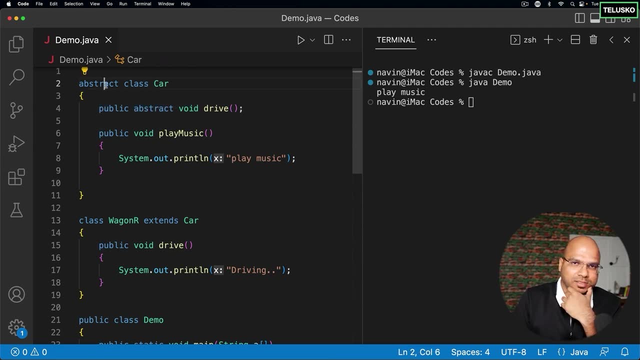 That's how you can create an abstract method And basically that's how you can restrict the creation of the object here. Now a few more points to remember. Is it compulsory to have an abstract method in the abstract class? I mean, we know that it is compulsory. 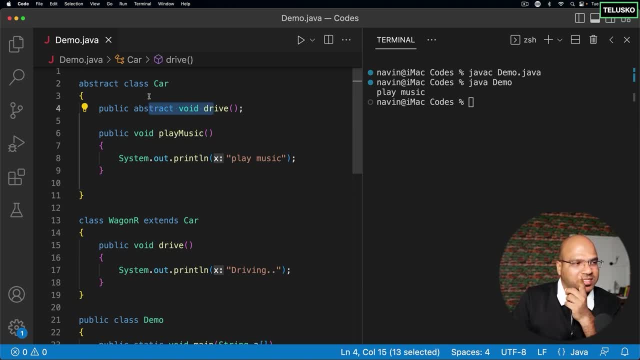 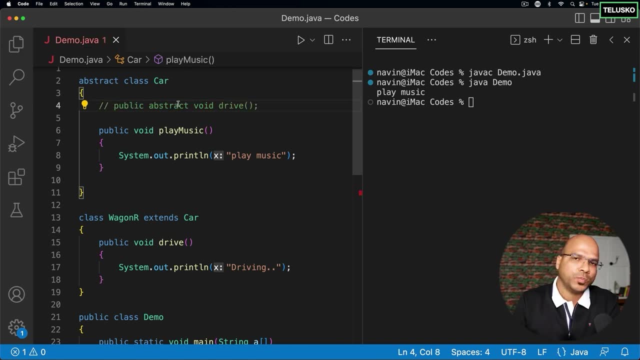 to have the abstract method. You need abstract class, right, But is it compulsory to have an abstract method in the abstract class? Let's do that If you come in this section. okay, you can see. there's no problem. It's not like an abstract class should have abstract method. 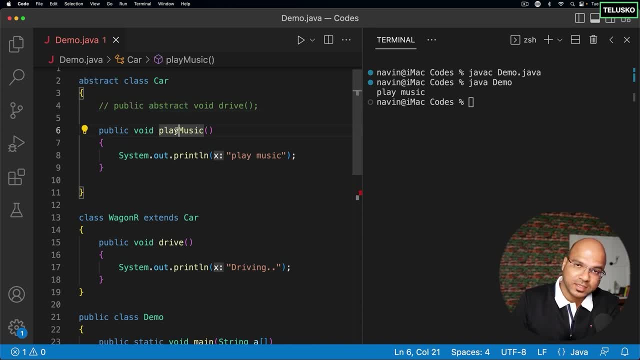 Abstract class can have abstract methods. It can have normal methods. So you can have an abstract class which only has abstract methods. You can have abstract class which has only implemented methods which are this, which are non-abstract methods, And you can have an abstract class. 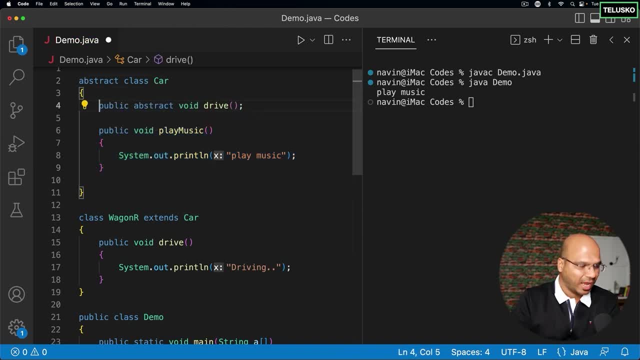 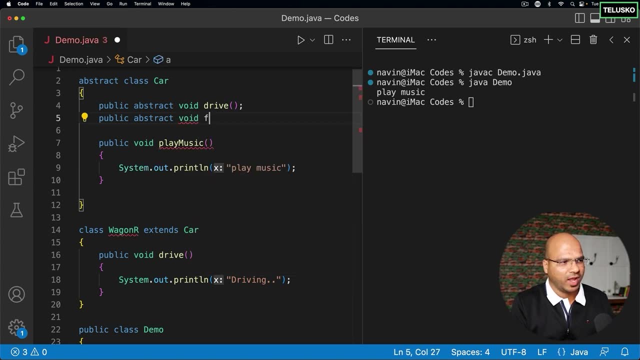 which can have both normal methods as well as the abstract method, And you can create multiple abstract methods. okay Example: if I can come back here and say, hey, you know, I want a car to fly. I don't know when this is possible. 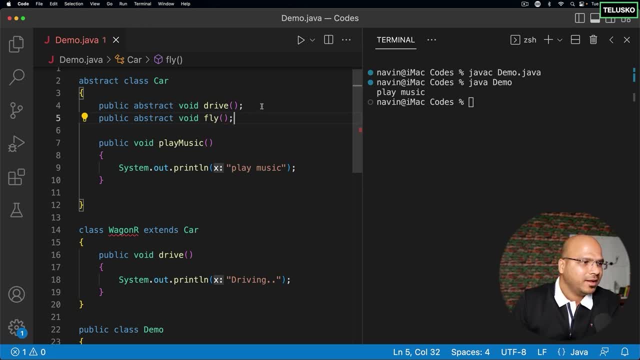 but in the movies you see that right. So a car jumps from one building to the other building. Okay, and I hope you know the movie name, But anyway. so if you talk about this abstract method which is fly- and you can see I'm declaring it here- 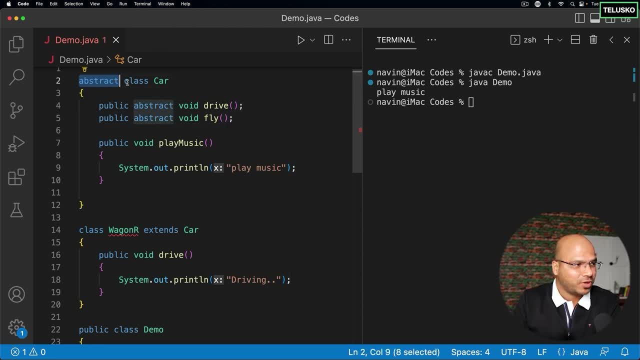 Now, when you declare a method and when you say you have an abstract class which is getting implemented or which is getting extended by another class, it becomes compulsory for you to define one more method here So you can say public, not abstract. 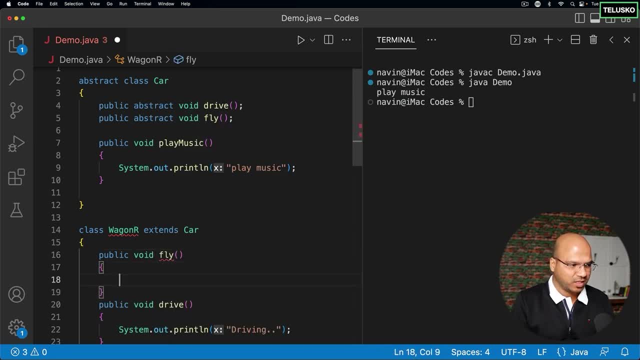 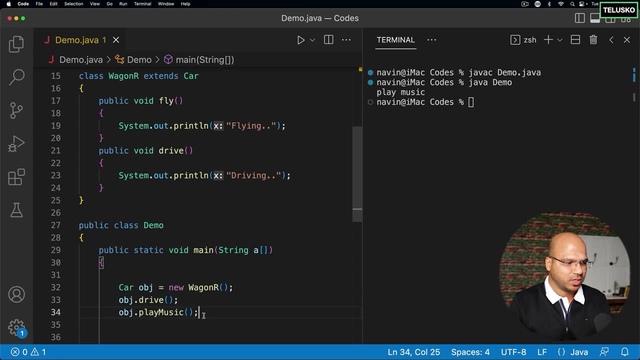 You can say public void. You have to define fly as well, otherwise it will not work. So you can say flying okay. And now with this you can call the methods, You can say objfly, and this should work. 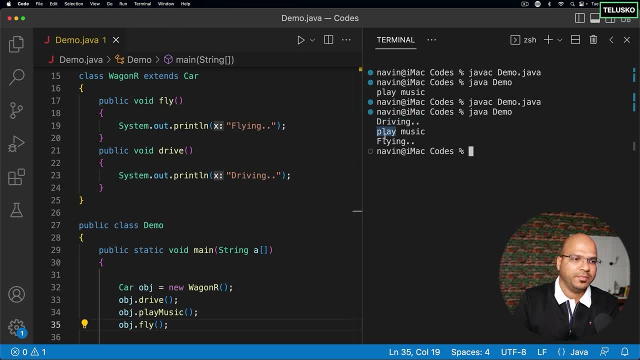 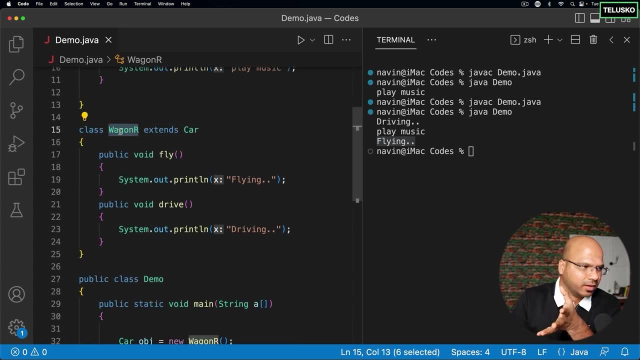 Compile run and you can see it says driving, play music and flying. Now there's one important thing here, which is what if, when you are creating this class wagonR and then you are not able to implement fly, what will happen? 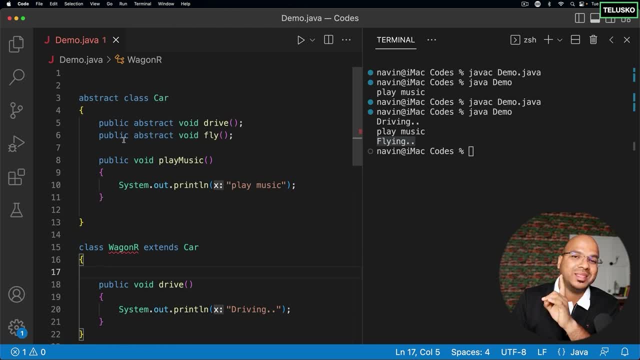 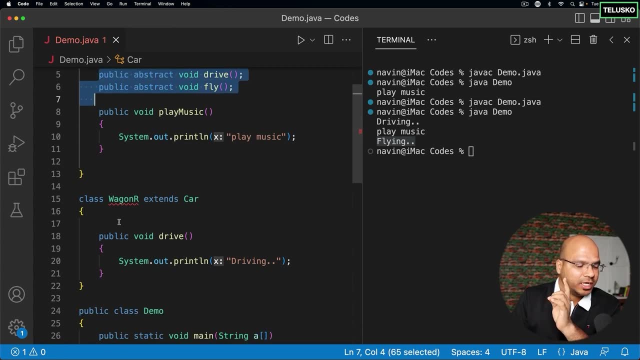 First of all, it's compulsory to define all the methods, Okay, all the abstract methods. So you can see, in this class we have three methods, but only two methods are abstract And that's why it says it should define fly as well as drive. 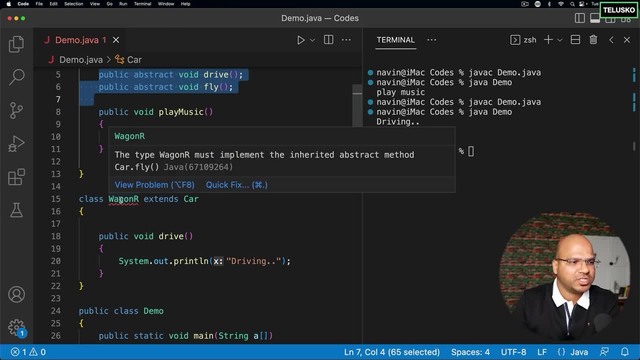 But we are not implementing fly. So you can see. it says the type wagonR must implement the inherited abstract method carfly. But what if you don't do that? So in that case, if you have a class which is not able to implement all the methods, 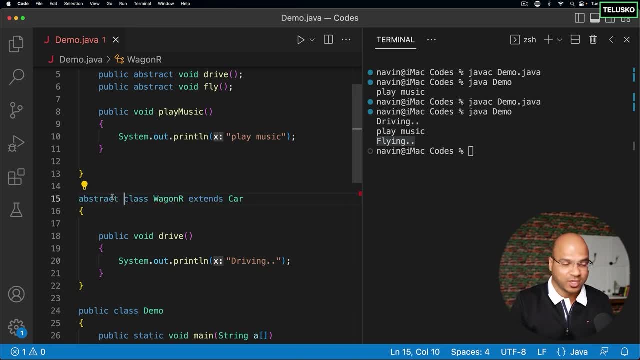 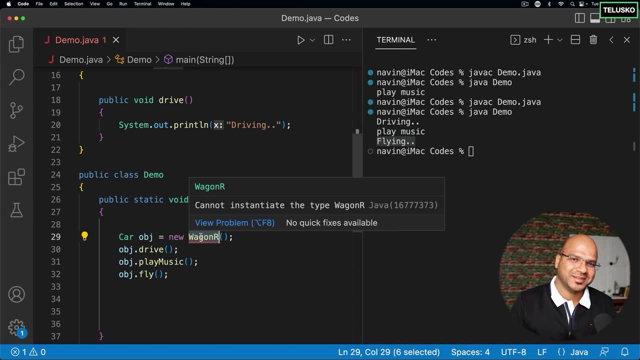 in this case, even this class becomes an abstract class. So you have to make it abstract class And you can see there's no error. But the problem now is you can't create object of abstract class, right? So maybe you have to create a new class here. 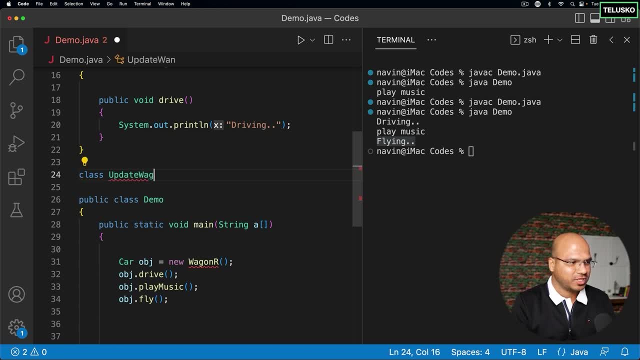 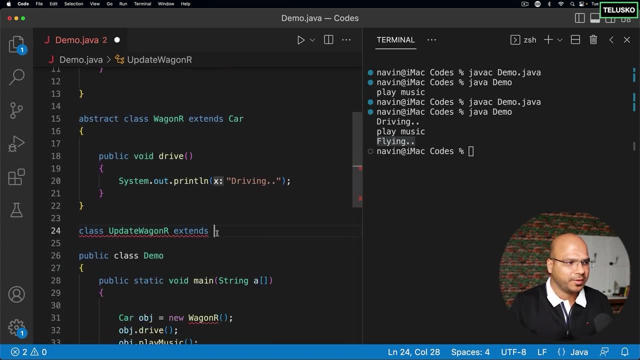 by saying: updated wagonR, which can also fly, And this will extend. Now, which class you want me to extend? The car or the wagonR? Of course, wagonR, right, Because you will get this drive feature from wagonR. 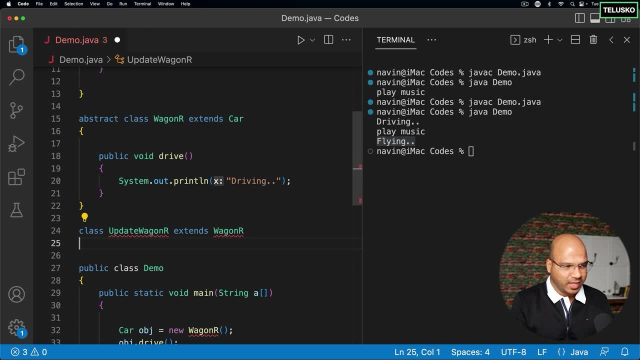 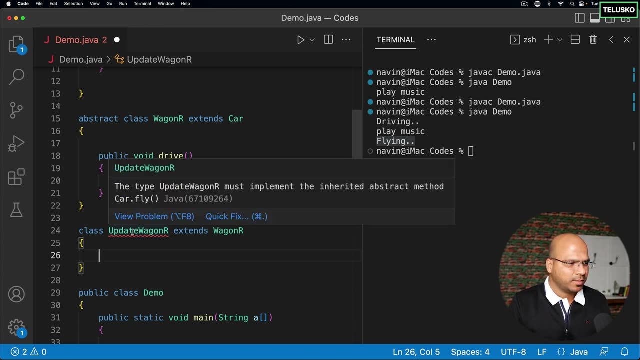 So you can simply extend it with wagonR And then here in this class you can basically create object of fly. In fact, if you are using IDE and if you're lazy to type, you can come to this error and you can say: fix, quick fix. 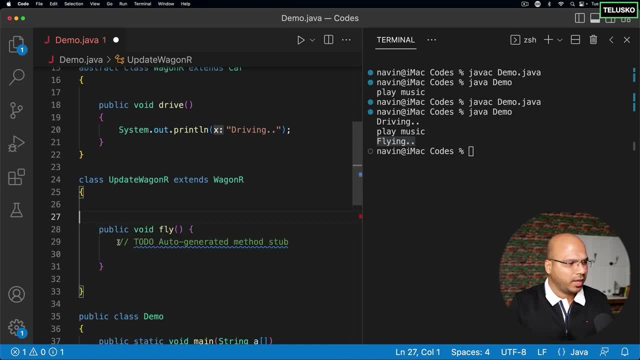 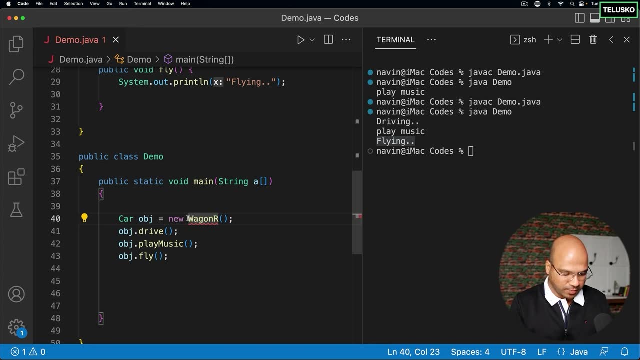 add unimplemented methods and it will do it for you. Okay, and here we can say flying, So even you can do that. The only thing is now: the object will not be of wagonR, The object will be of wagonR. 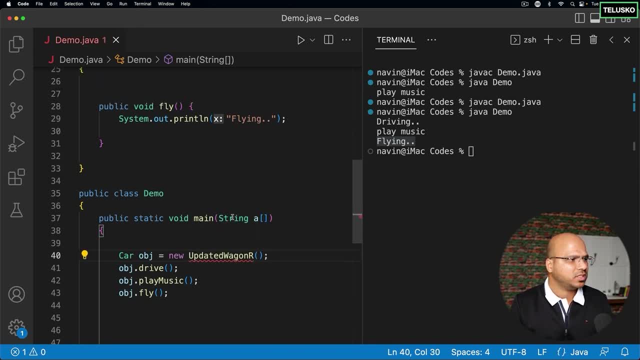 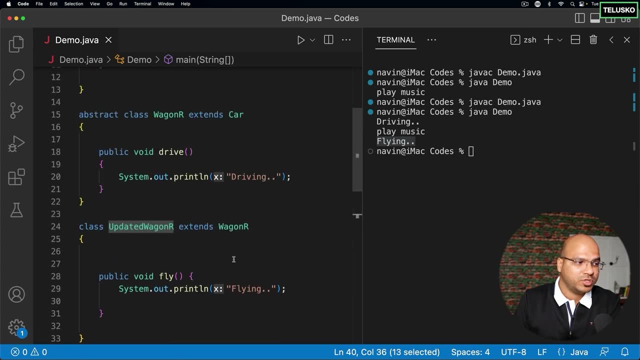 The object will be of updated wagonR. Is it the method class name? Okay, it should be updated, right. So that's how you can create a object. So again, we are not getting object of abstract class, We are creating object of the class which is not abstract. 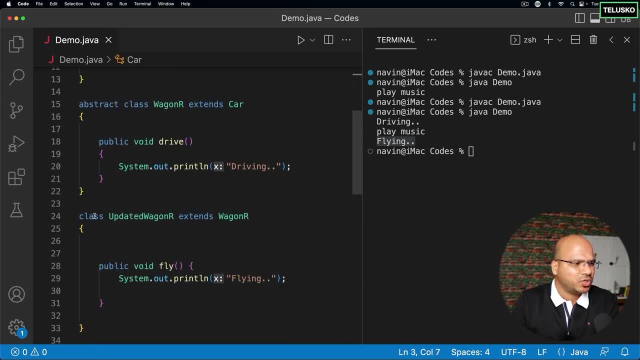 Okay now, since we are calling this class as abstract class, even this class should have a name, right? So normally we call them as a concrete class, So we can say: this is a concrete class. Okay, so we have abstract class and then we have concrete class.